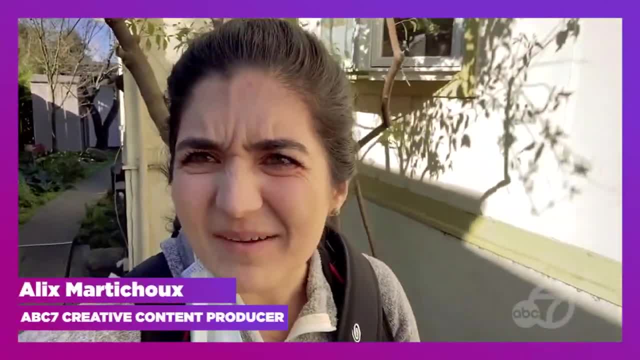 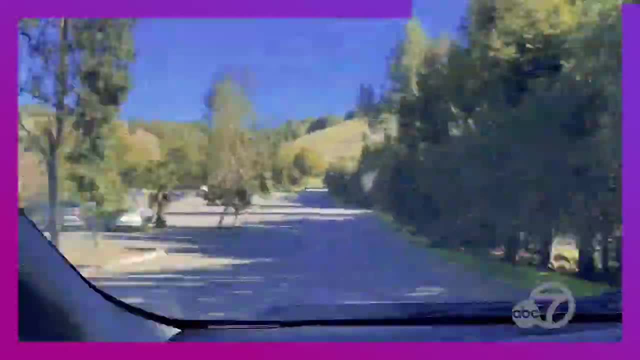 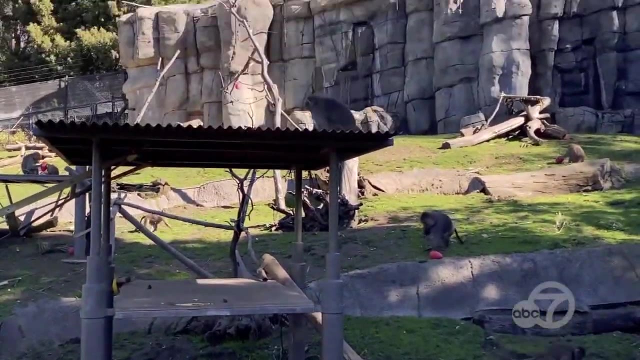 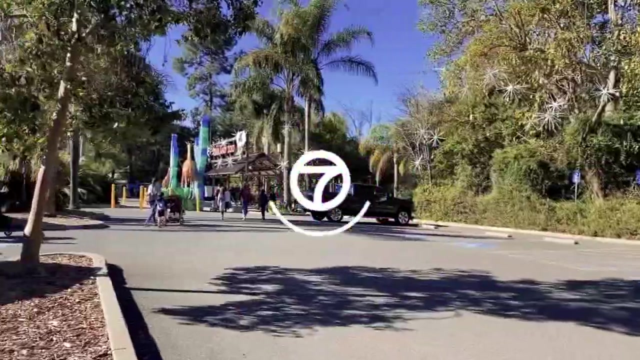 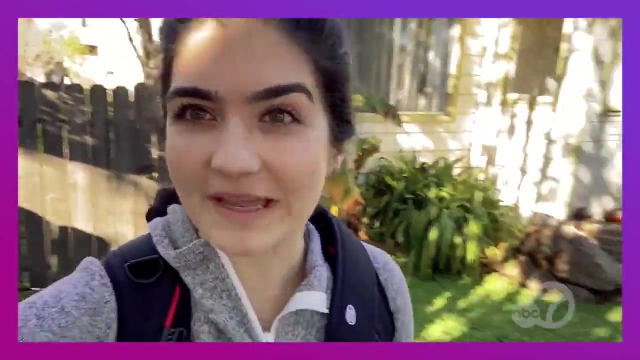 Heading out. today I have the best assignment in the newsroom. I'm going to the Oakland Zoo- Beautiful day for a zoo visit. They're going to show us some behind the scenes stuff that most visitors don't get to see, and I'll show you. 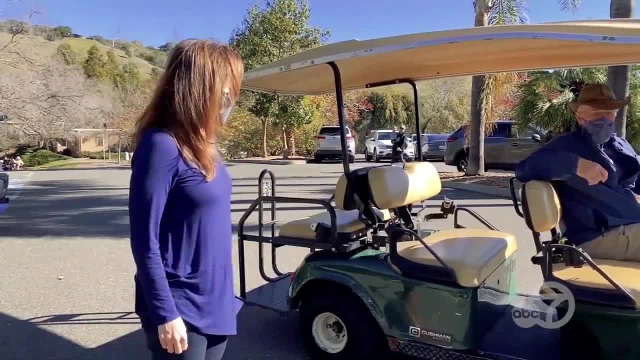 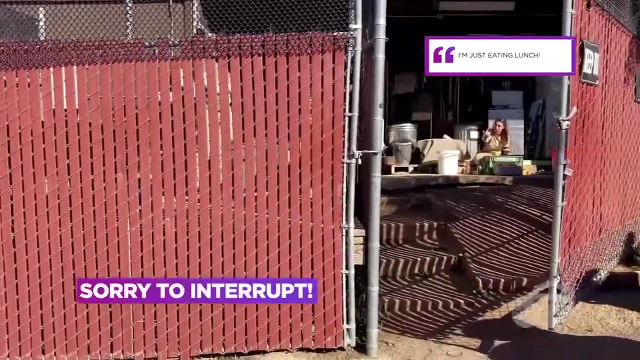 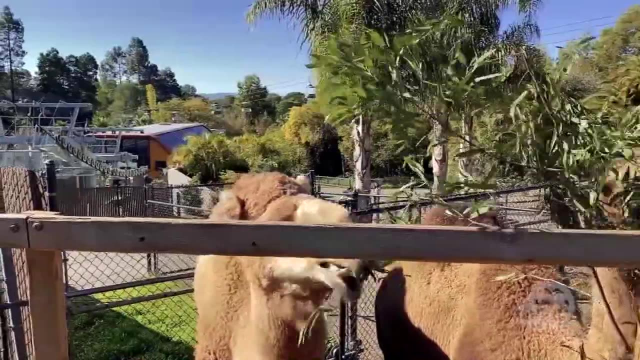 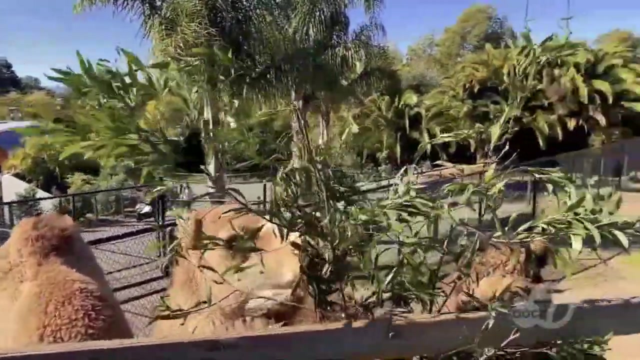 Hi, Is this our ride for the day? Is this a good time Get a picture of her eating lunch? Here we have Bahir- He is the only male- And then we have Zahara Layla and Sabah Green. 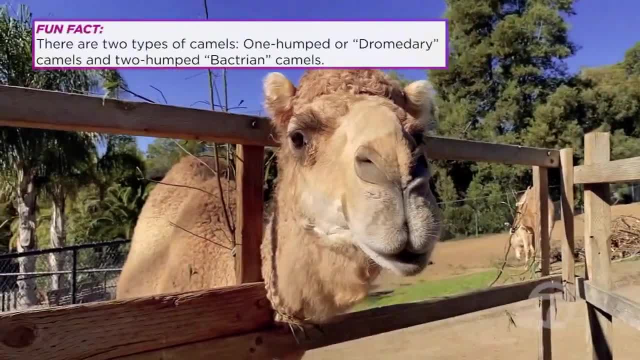 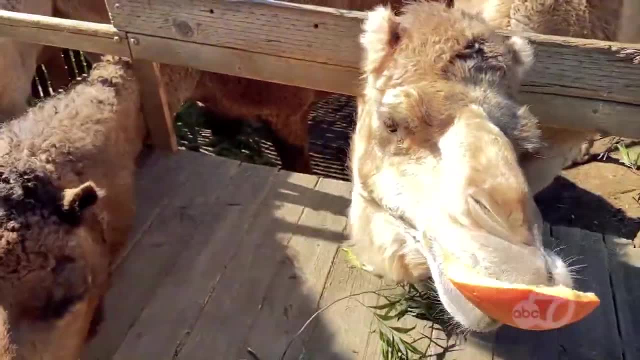 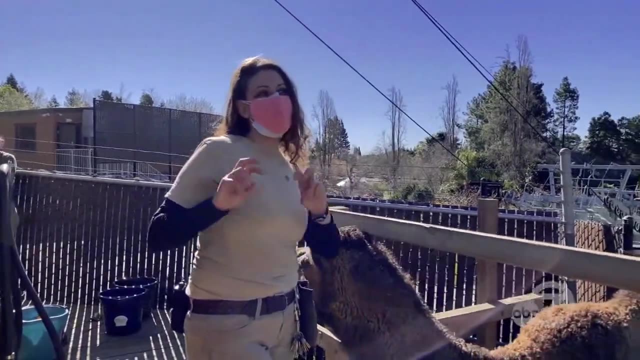 We like salad, Hello friend. So Zahara and Sabah and Layla, they really like bananas and pumpkins and all sorts of stuff, But Bahir always says we need a salad. That bucket's empty. We don't say that they're sweet, we don't say that they're mean, we just know that they have a ring. 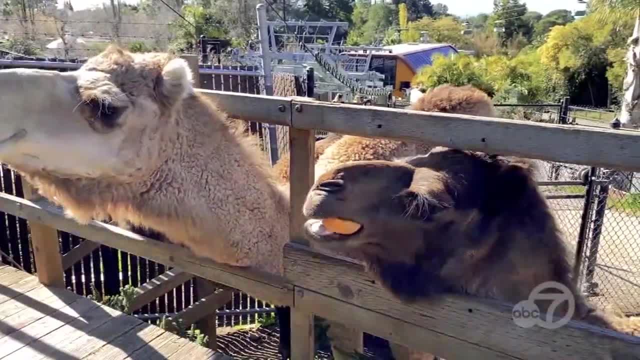 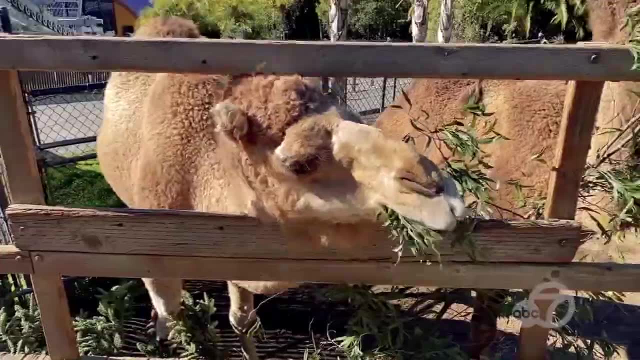 Mmm. But you know camels are very smart, charming animals. They are pretty cool. I feel like I love camels now. You don't think you come to the zoo to see the camels, but you fall in love with them when you're here. 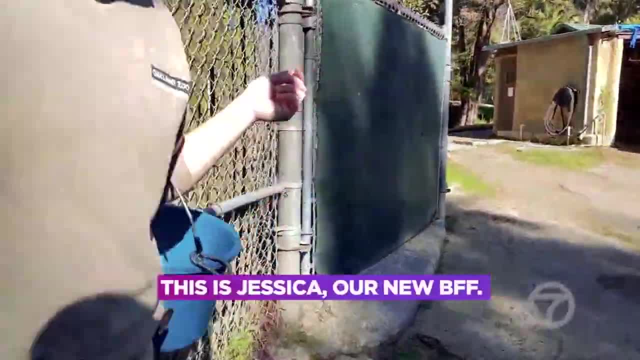 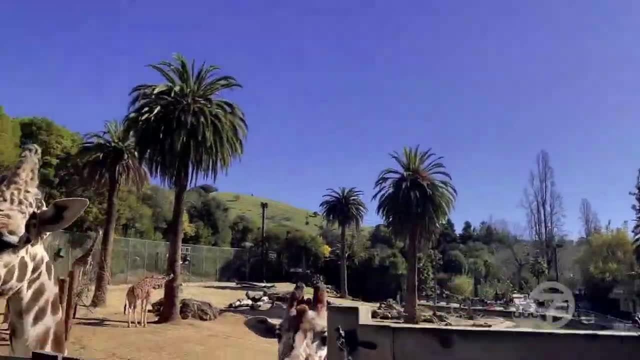 All good. Hi, I'm Alex, Hi, I'm Jessica. Nice to meet you, Nice to meet you. Oh, someone's waiting for us. Oh, always, Who's this? So this is Mabusu, His name, Mabusu means kisses in Swahili. 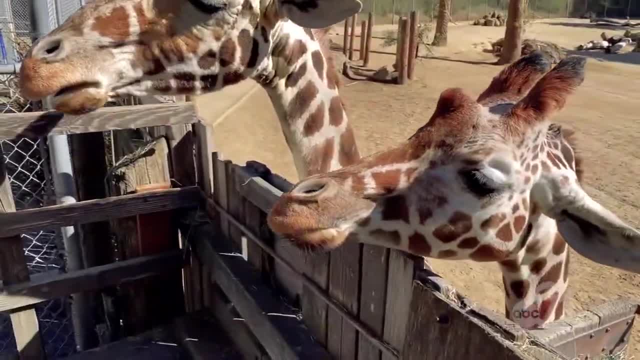 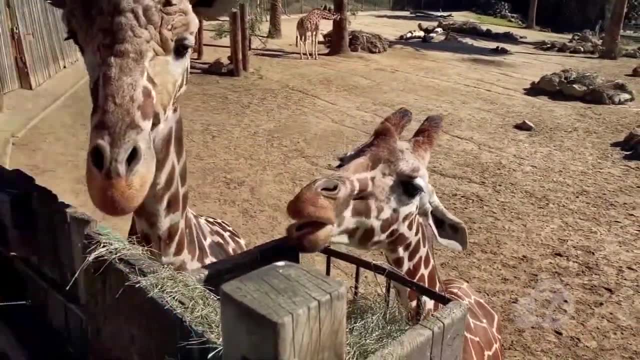 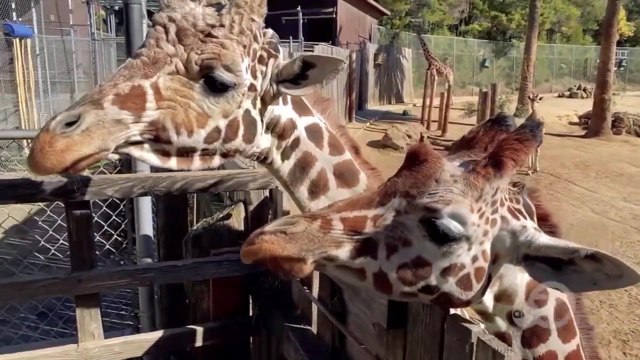 That's very apt. This is actually his daughter. Oh, Maggie, Hi Max, Nice to meet you, Maggie. She was born here And she turned nine in January. Maggie's a much more delicate eater. She is A little less intense. 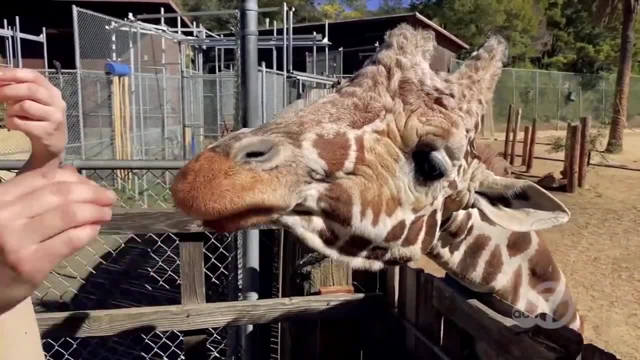 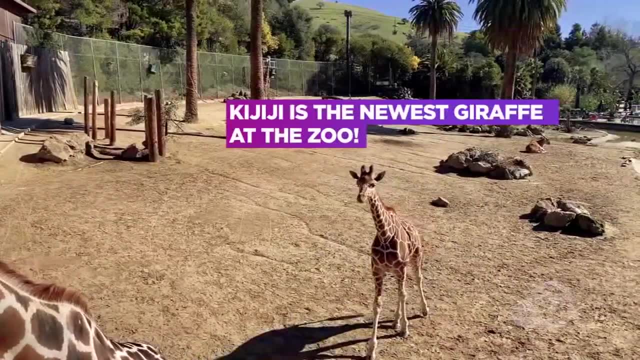 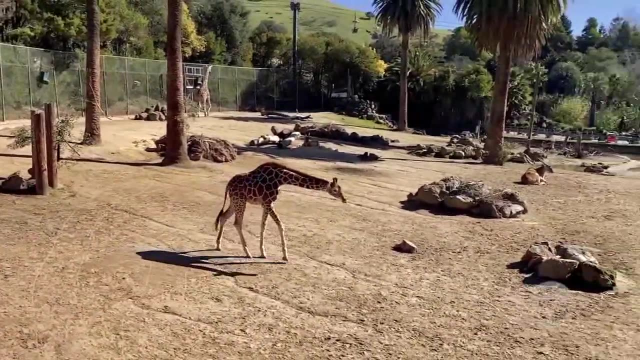 Mabusu has a very aggressive tongue, I would say When feeding. But Maggie's very sweet Kijiji, Yeah, Come say hi, And Kijiji means village in Swahili, And she's really confident, She does not get very nervous. 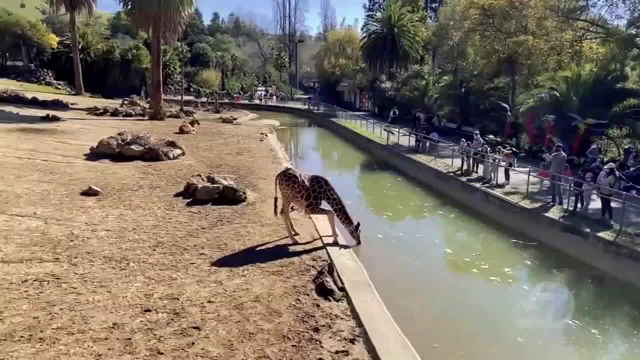 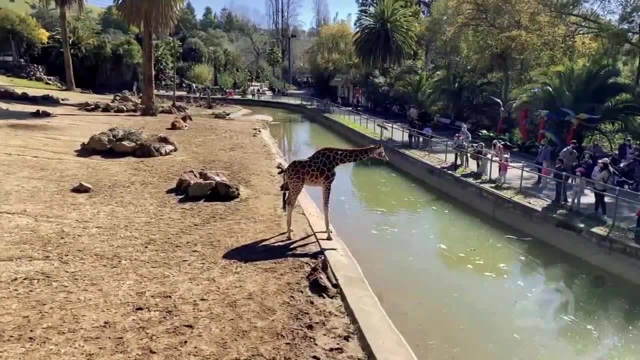 She's very curious. She gets along with everyone. She gets into antics, though for sure Any other juvenile would. Oh, I like to refer to that as the splash zone. Oh my, Oh my, Oh my. 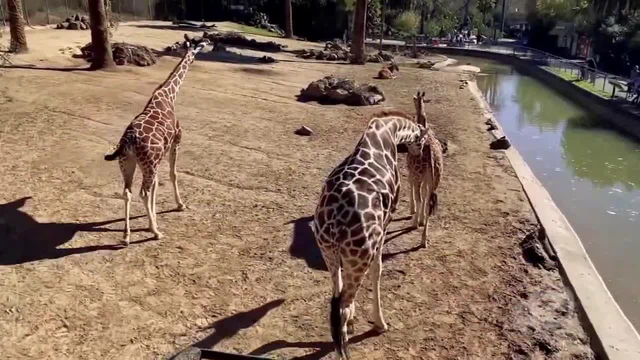 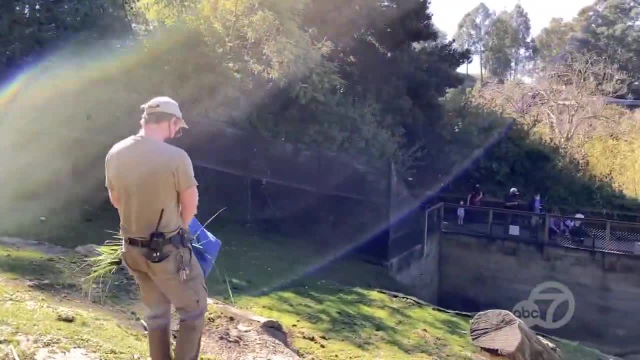 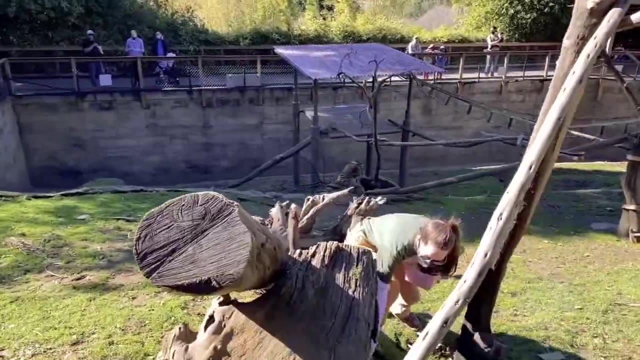 That's you being a big guy. Oh my, everyone. I'm standing inside the baboon exhibit. Zookeepers are setting up food, hiding it all over the place so that when the baboons get released they go on a little treasure hunt. 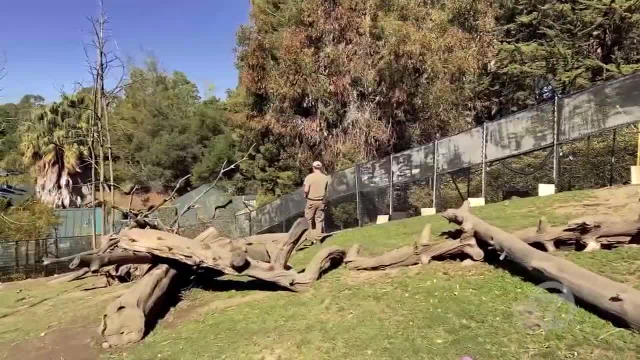 But they're going to get me out of here first so that I don't get too behind the scenes and too involved. You'll see, when I open the door, all 15 will come in. Oh my gosh, Oh my gosh. 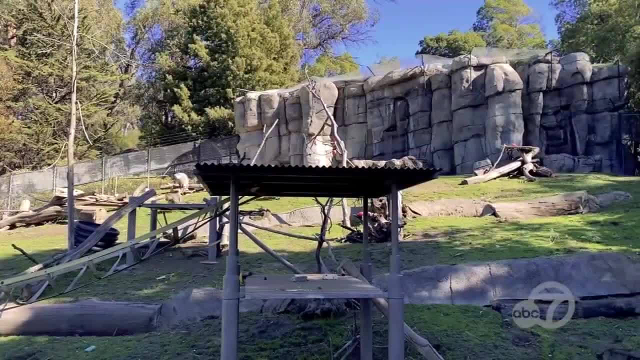 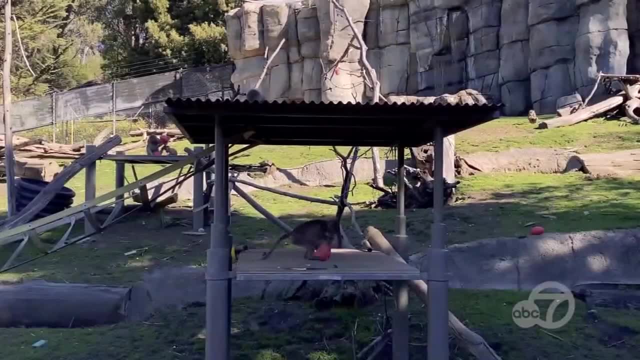 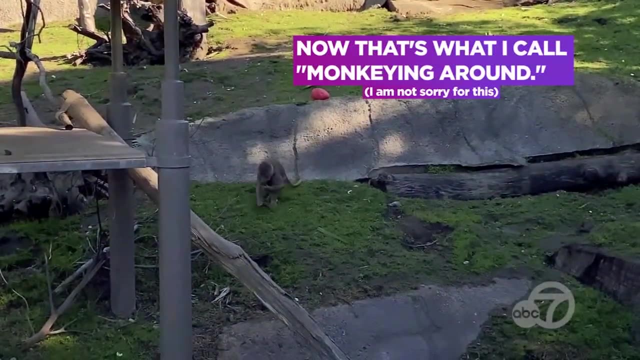 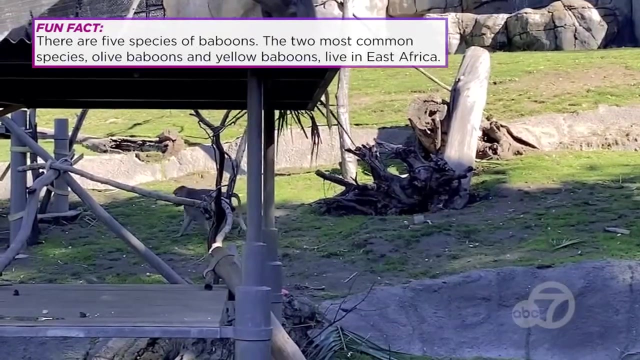 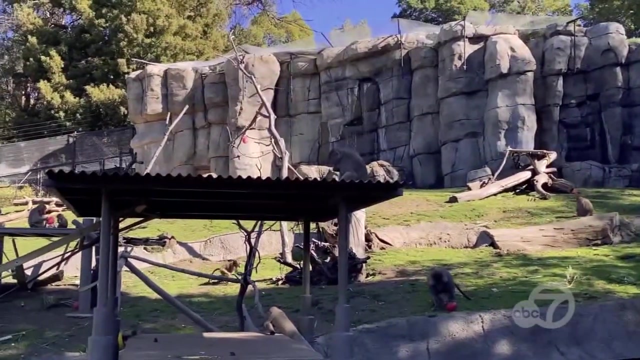 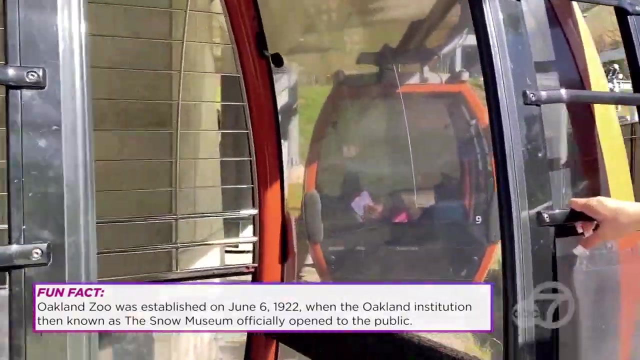 All 15 will come flying out at once. Oh wow, Oh, they look pretty happy, They look super excited. That's so cool. Oh wow, Hi guys, Thank you, Thank you, Thank you. Have a nice ride out. 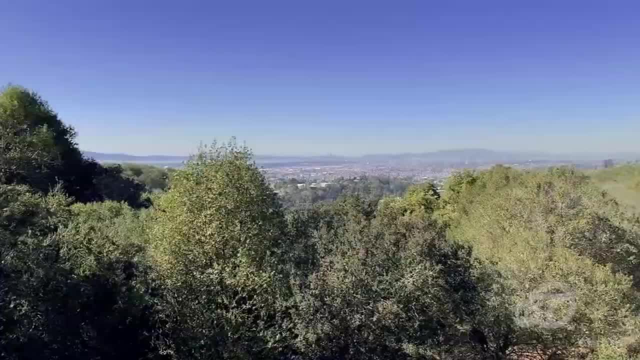 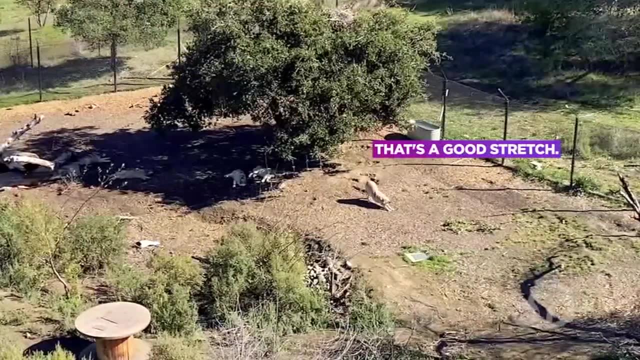 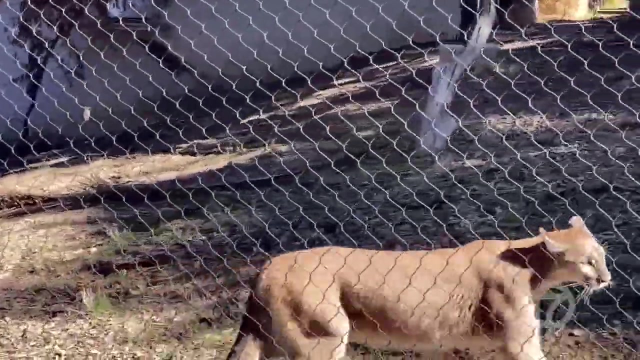 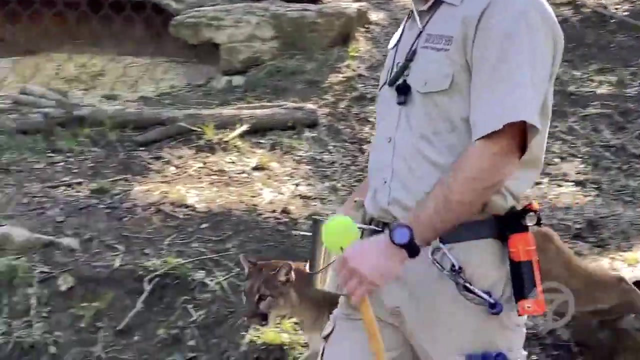 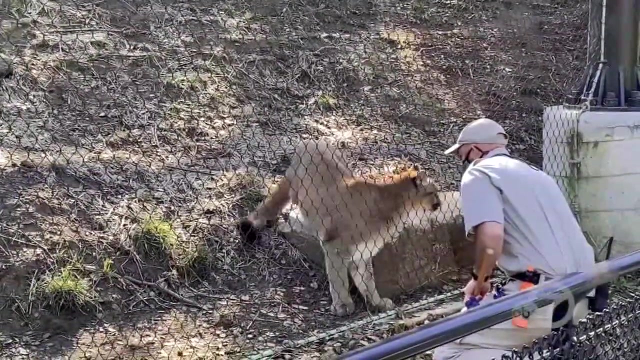 Thank you. How do you not just stand here all day? Come on, These behaviors do have a purpose behind them. It's not just tricks or something like that. We're using the ball targets to be able to help, to direct their bodies and be able to put them in positions. 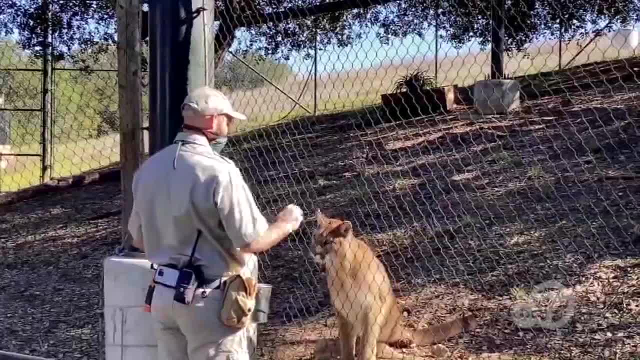 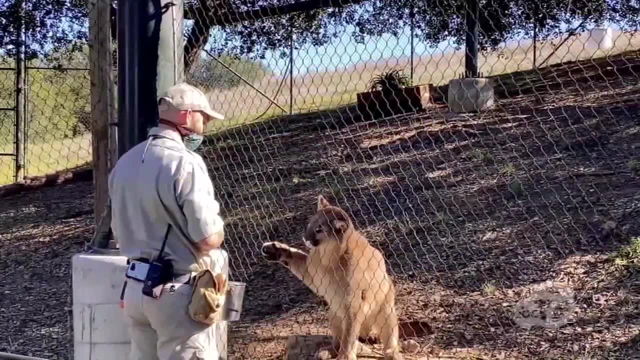 where we can look at them really well. pause, while it looks like a high five, is actually so we can check their feet, make sure that they've got healthy pads and everything's working well. And then Coloma and actually all three of our cats. 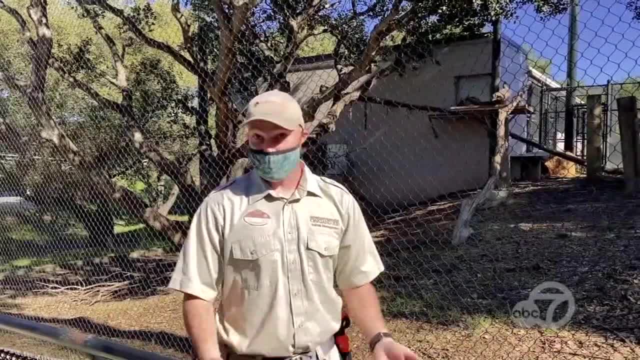 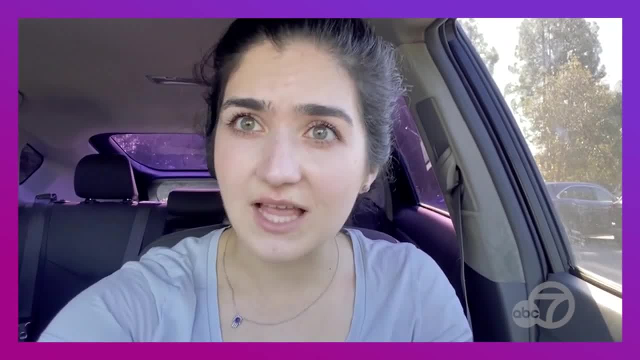 all are trained for voluntary injections so that we can actually give them vaccines without having to dart them. So it's much less scary for them, which makes it a lot easier for us too. Great day, What a great day Inside, behind the scenes. 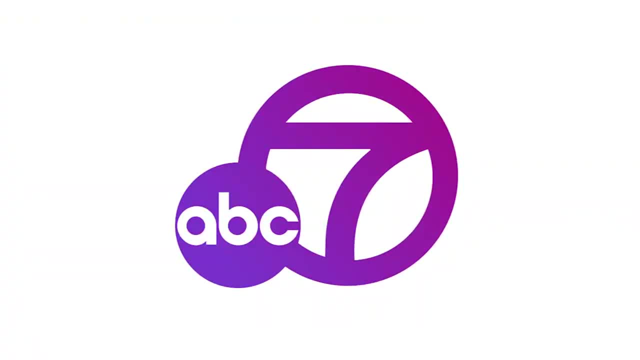 Can't imagine a better assignment than that. We'll be right back.